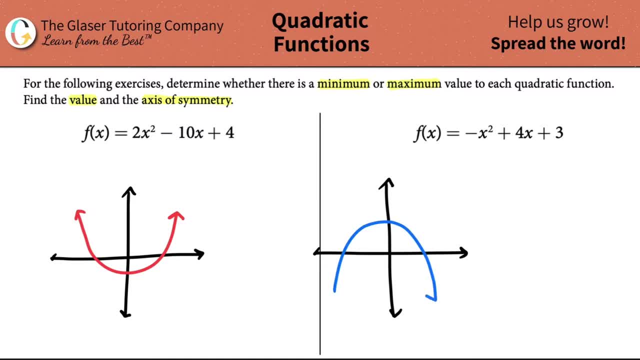 Oh, or they're frowning at you, okay. So they're very simple. They're either going to be smiling or they're going to be frowning. Now the turning point, which is called the vertex. how I drew it, the vertex would be right here. It's the turning point between going like down. 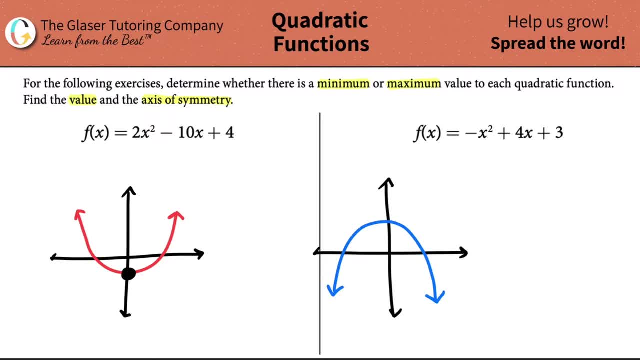 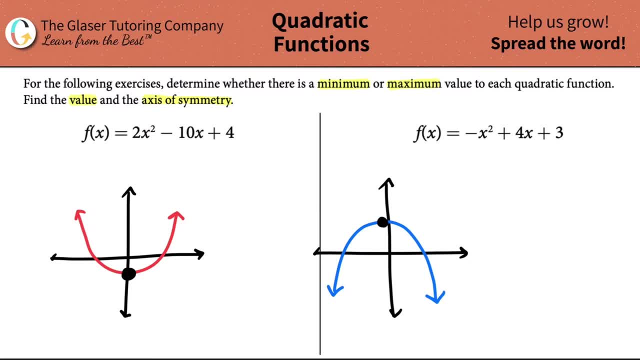 Okay, Okay, okay. okay. The way that I drew it kind of looks like over here. right, It splits the graph into two components: one that's decreasing on this side and one that's decreasing on this side, And the same thing goes. 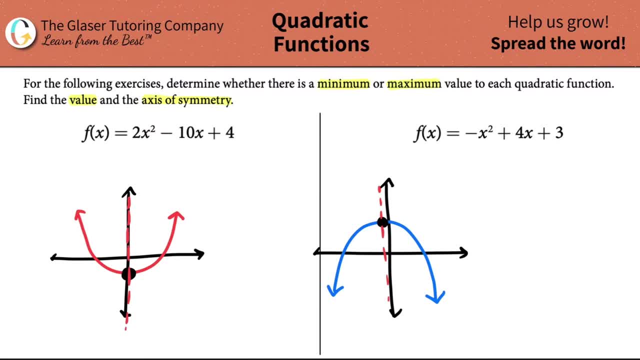 for this one as well. right, So the vertex is a huge component of our quadratic formula. Now just know that when you're smiling, the vertex which is a point will be the minimum value of the graph. right, You can't go any lower than the vertex. So when you're smiling, or when the 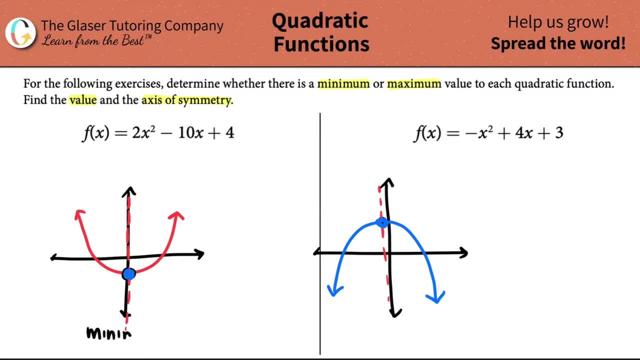 quadratic is smiling. you will have a minima right, Or it's called the minimum value, whichever one you want to say, The frowny one, and I'll say that over here, this is smiling smileys, this is frowning The maximum. well, I just gave it away. right, The vertex is the highest. 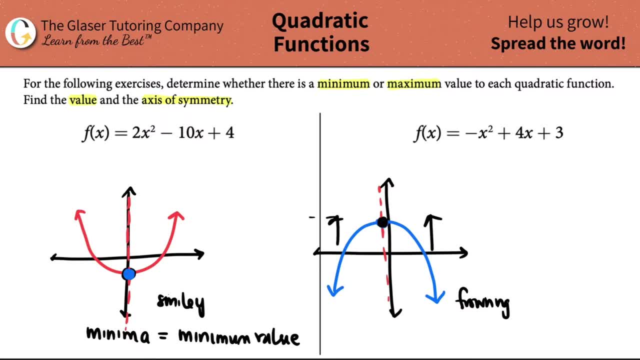 portion of the graph right Can't get any higher than the maxima. So if you have a frowning quadratic function, you have a maxima or a maximum value. Sorry for my terrible handwriting, I'm just trying to write fast, Okay. 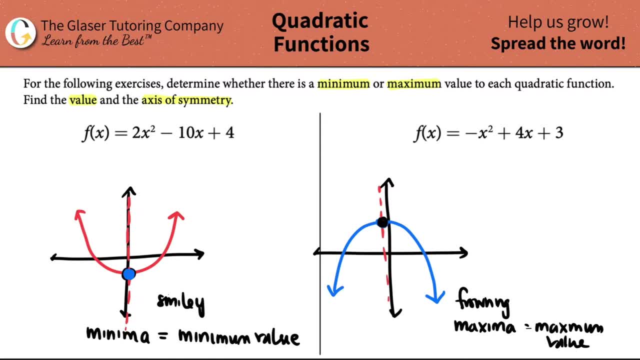 Now, how do we know if a graph is going to be smiling or frowning at us? The answer lies in the A value. okay, And it goes with the context of smiling versus frowning. If you're smiling right, you're happy. I mean, you know in a very general term, right? So smiling is positive. 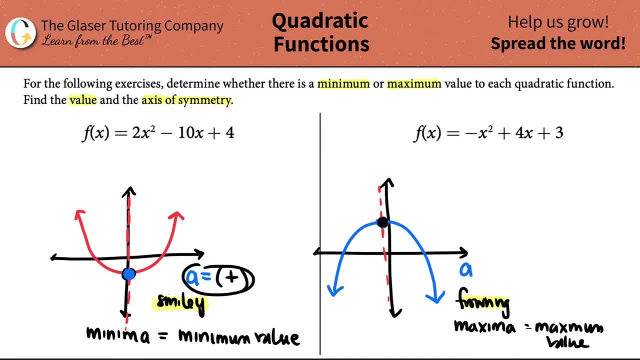 right, You're positive, you're smiling, So my A value has to be positive here. Frowning negative, sad, that goes together. And remember the A value is always in front of the X squared value. So in the first example my A value is equal to two. It's a positive value. 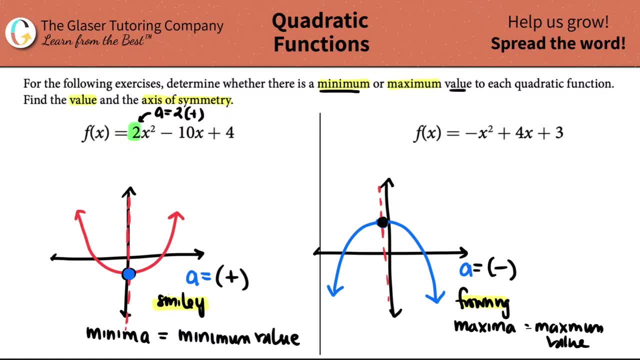 So I know that I'm going to have a minimum value. It is this type of graph: It's a smiley face, Okay, So now the whole thing is that we need to know what the value is and what the axis of symmetry is. Okay, So I'm going to have to erase these graphs, because now I'm going to have to do the 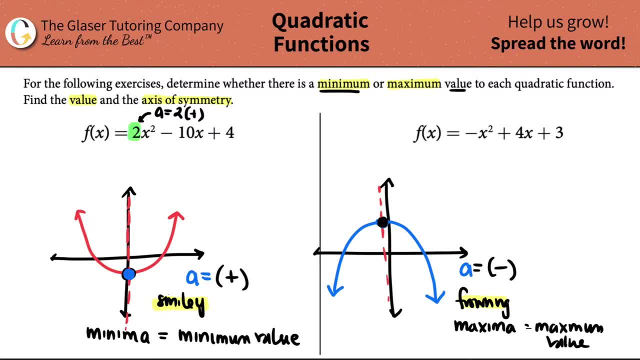 algebra right. So if you want pause the video, write this down. but I got to get rid of it, unfortunately. Oh, I hate to see my work go, but that just leaves more room for more work, Okay, Okay. So now we need to find that value. 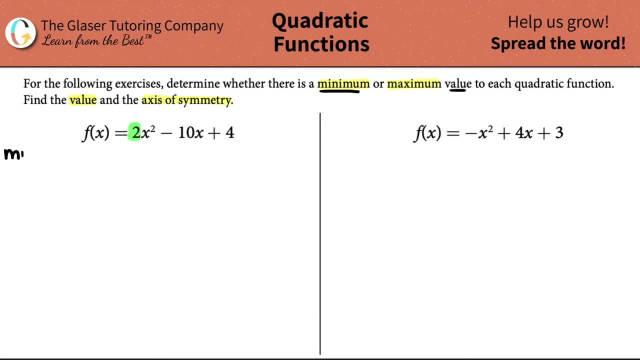 Of the minimum here, Minimum value. And how we do that is by going by what that vertex is. Now remember a vertex. the standard form is H comma K right. The value of the minimum is always going to be your K value. 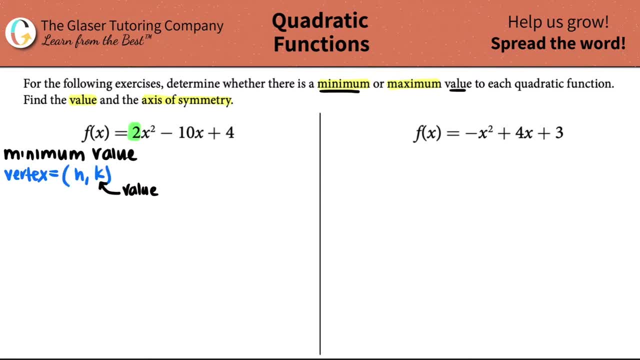 mainly because the value of the minimum is going to be your K value. So if you're going to have a, the K, if I turn this into X comma Y, the Y axis gives you the highest point or the lowest point, the max or the min, So the value of the minimum will be the K value. The axis of symmetry is the. 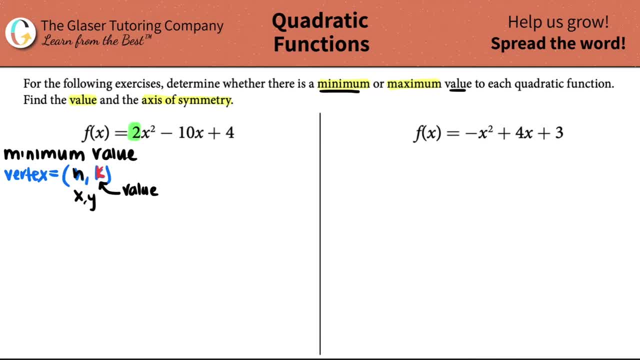 other guy- The axis of symmetry is H, So- and I'll put that in quotes here, because there has to be something that we have to do- to get the K value- So the value of the minimum will be the K value When we state what the axis of symmetry is. but I'll tell you when we get there, So just know that. 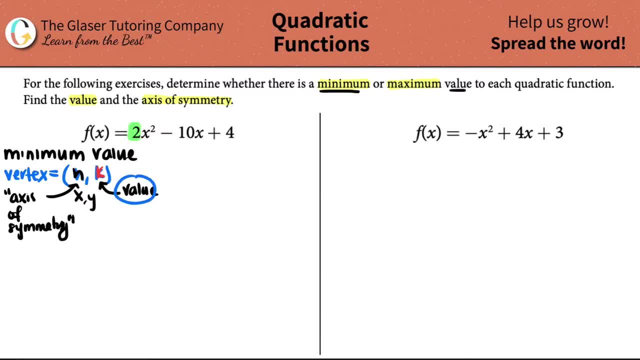 in. in general, the K value is going to be that value of the minima. The H value is the axis of symmetry. So now, how do we get H and K? Well, remember, we've done tons of problems where we have been finding H and K, So we're going to run through it right In order to find an H and 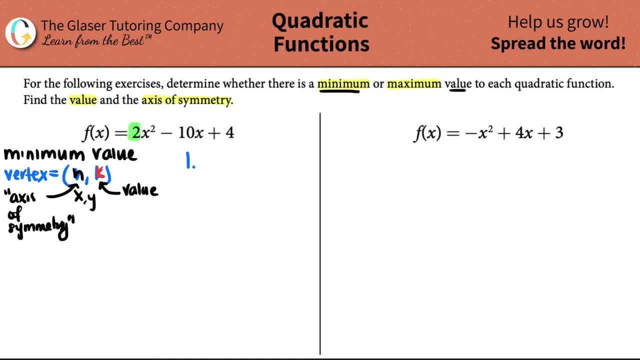 you'll always find an H first, And you could think of it like that way because you know H comes with 4K in the alphabet. Remember that H just equals negative B divided by 2A. I have A, B and C values here. 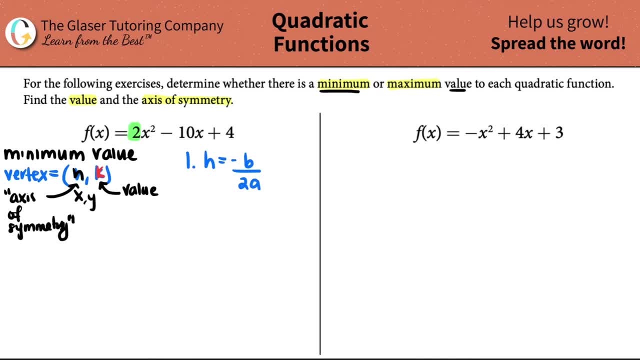 So let's just quickly go over it. I have a 2,, I have a negative 10, and I have a positive 4.. So my A value is 2,, my B value is a negative 10, and my C value is 4.. 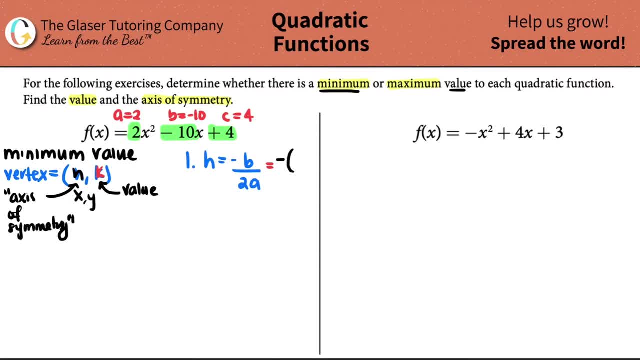 So I'm just plugging in my values: negative B, which is a negative 10, divided by 2 times 2,, 2 times A, right? So I clean this up, This would be 10 over 4.. And if I just simplified, right. 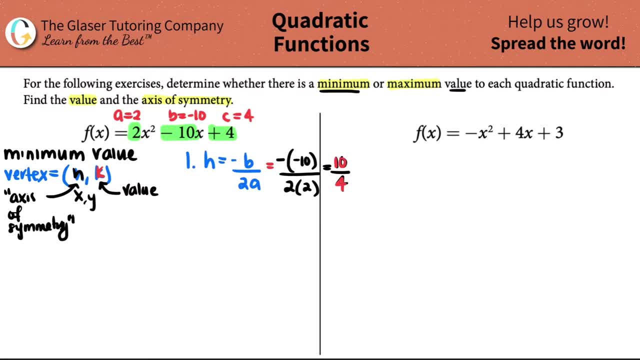 what number is common between 10 and 4? A, 2.. So 4 divided by 2 is 2.. 10 divided by 2 is 5.. So I have an H value of 5 over 2.. Remember, this is the axis of symmetry. 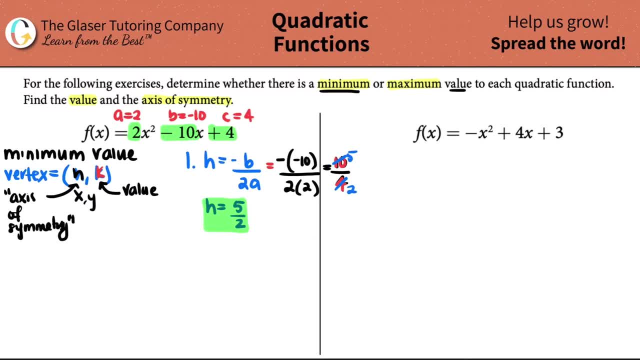 Now, remember I said that I have to, you know, tell you a little bit more context for axis of symmetry. When we're saying that it's an axis of symmetry, I can't say H. Technically it's incorrect. But remember, H is the same thing as X And since a graph is based off of X and Y's, 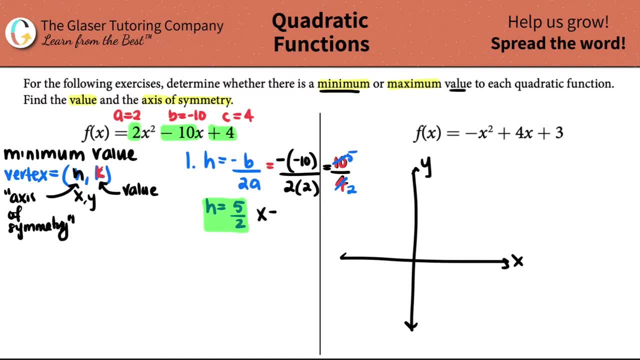 that's why you have to say: my axis of symmetry is X equals 5.. 5 over 2.. Technically, if you say the axis of symmetry is H equals 5 over 2, I would have no idea what you're talking about, because the graph is X and Y, So that we found the first part This: 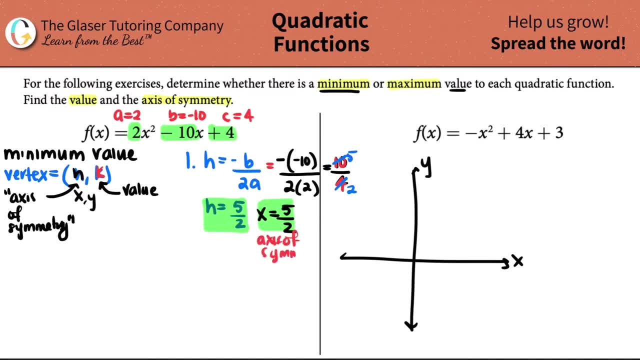 is the axis of symmetry. Now, what this actually means in context is if I go over on my X to 5 over 2, so let's just say that I don't know, it's somewhere over here, right, That is the turning. 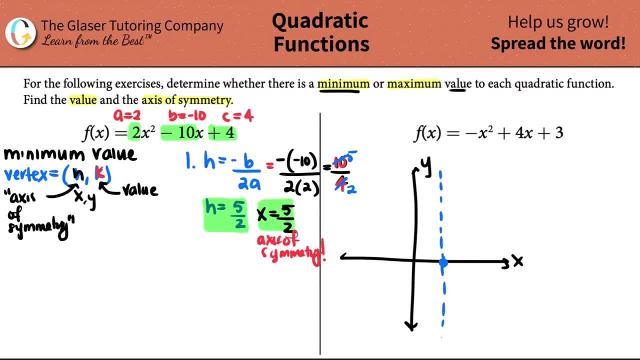 point of the graph. So if I go over on my X to 5 over 2, that is the turning point of the graph. Now we already discussed that we're going to have a minimum value because this is smiling. But now, 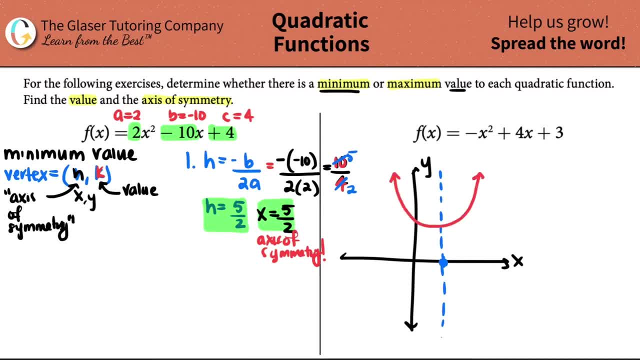 here's the question: Is my graph like this? Well, actually, let me make it a little bit right, Because that has to be the turning point. Is it like this? Is it like this Right? Is it like this? 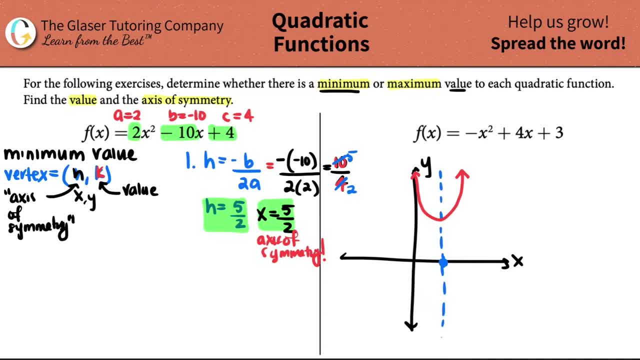 We don't know what that max or min value is yet. right, My min value could be all the way up here. It could be maybe- Okay, It could be at the origin, I don't you know. Or it could be at the bottom. So yeah, Let's find. 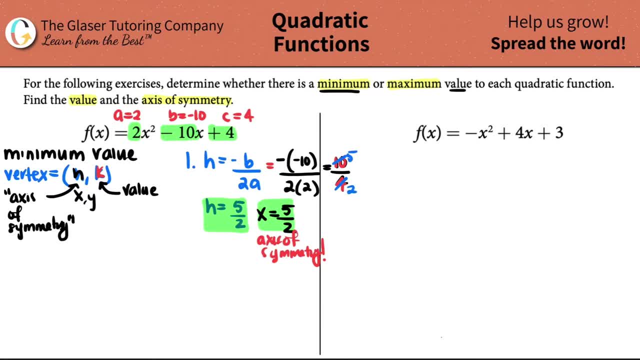 out that value And remember that's the K value. So the second thing that we have to do is find that K value And remember the K value just equals F of H. What you're going to do is you're going to plug in the H value into the formula, So instead of it being 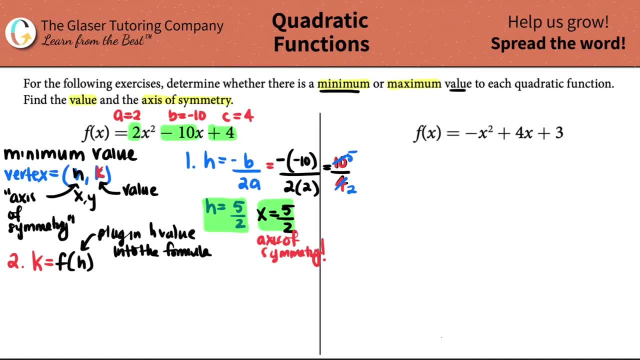 2X squared minus 10X plus 4, I'm going to plug in my 5 over 2 for all of my X values. So it was really 2X squared minus 10X plus 4.. But now for all the Xs I'm going to input And I'll put over. 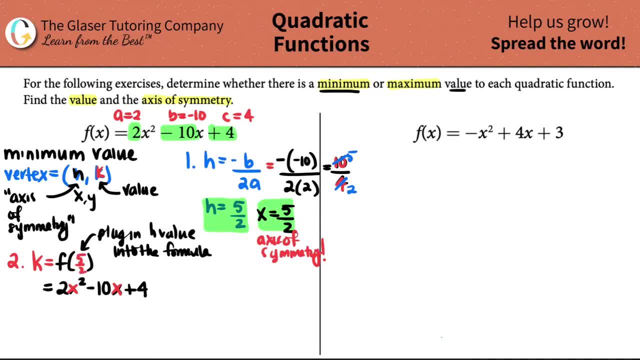 here That was a 5 over 2.. So if I color code this it would be 2 times 4.. And I'm going to plug in 5 over 2, and that's all squared minus 10, times 5 over 2,, plus 4.. 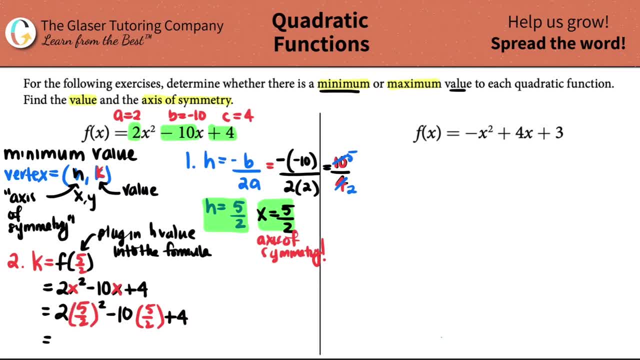 So let's get it done. We first got to do the exponent 5 over 2, times 5 over 2, that's x, that's, you know, 5 over 2, squared, multiplying fractions. I multiplied the numerator, I multiplied the. 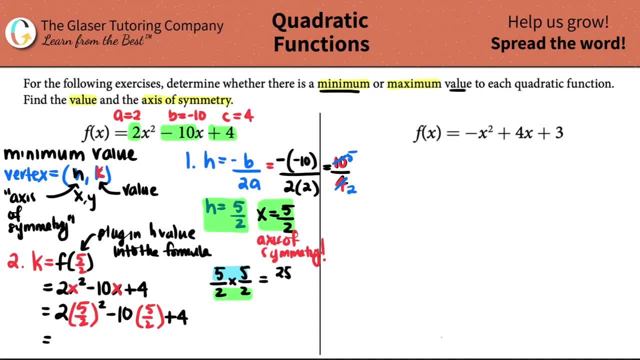 denominator. so 5 times 5 is 25,, 2 times 2 is 4, so this would be 2 times 25 over 4.. Okay, let's keep it moving. I have 10 times 5 over 2, I can simplify this. I have a 2 on the bottom, 2 and 10, are you? 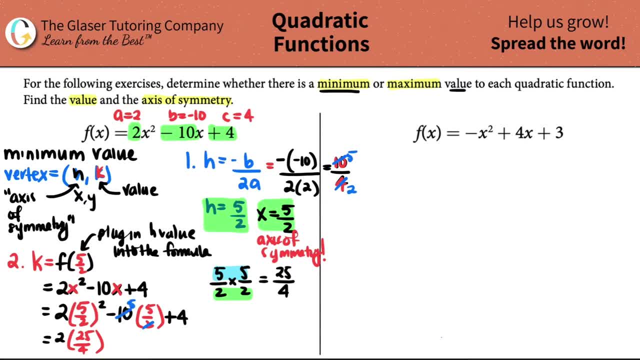 know common right: 2 times 5 will get me 10.. So now I just have 5 times 5, which is a 25,. so minus 25, and then plus 4.. Let's clean this up, right. 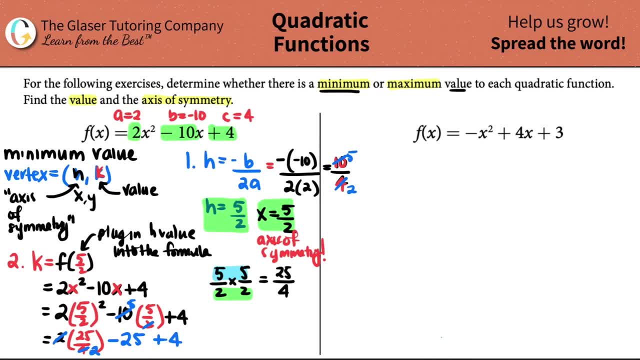 I have a 2 in the numerator, I got a 4 in the denominator. 2 times 2 is 4, so this would be the same thing as 25 over 2.. So now I have- if I can just get rid of this- I can say that this is 25 over 2.. 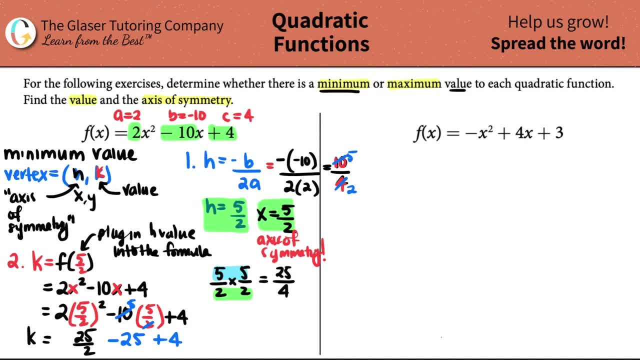 Now at this point, remember this still equals k. I'm trying to find that value, the minimum value, 25 over 2 minus 25 plus 4, you can just plug this into the calculator. I just like to work with fractions. it kind of gives you guys, you know, being more comfortable with fractions. 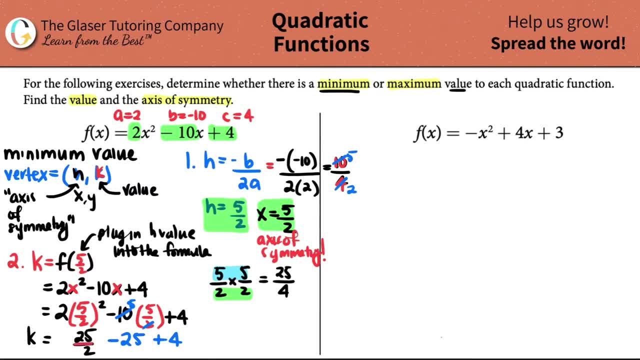 So I want to turn this into a common denominator. I see that my only denominator is 2, so I want to make all of these over 2.. But remember, they're over 1 now, right, Both of these. So what would I have to do? 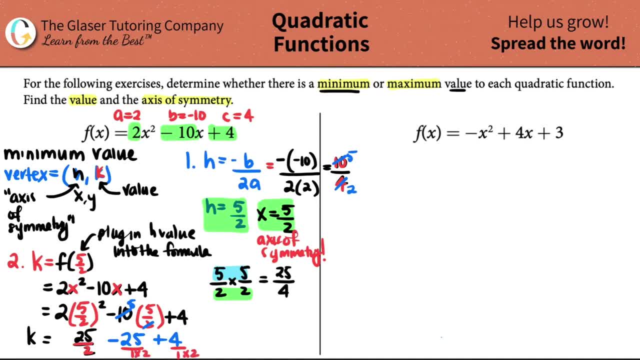 Well, I would have to multiply by 2.. But I gotta be fair. whatever I do to the bottom, I gotta do to the top. So this would be 25 times 2 over 2, 25 times 2 is 50, right. 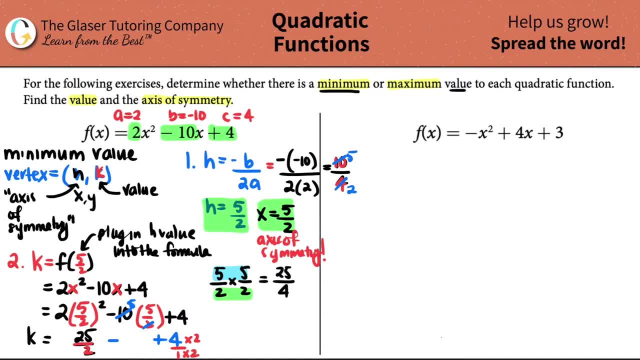 So I can just say that, instead of saying minus 25, I can say that this is minus 50 over 2, 25 divided by 2 is 25,. 50 divided by 2 is 25.. And then 4 times 2 is 8 over 2.. 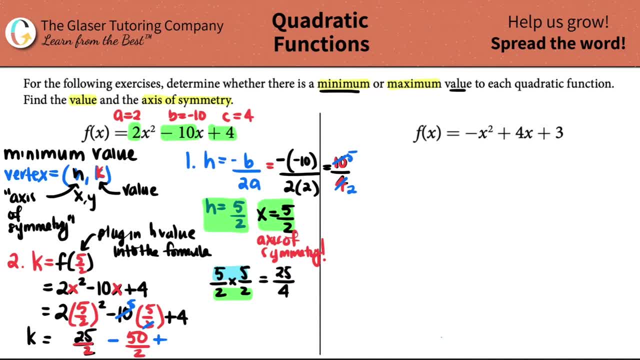 And then 4 times 2 is 8 over 2.. So instead of saying 4, I could say 8 over 2.. And remember, when you're adding and subtracting fractions, you only do the adding and subtracting on the top. you keep that denominator by itself. 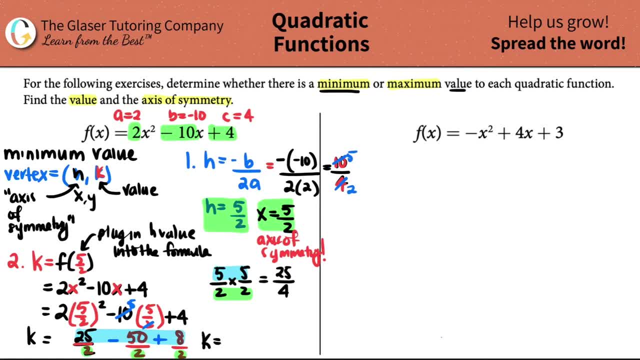 So the k value, which is the value of the minimum, would be 25 minus 50,. this is a negative 25, right Plus 8. This is all over 2.. So negative 25 plus 8, let's just do that quick. negative 25 plus 8 is a negative 17.. 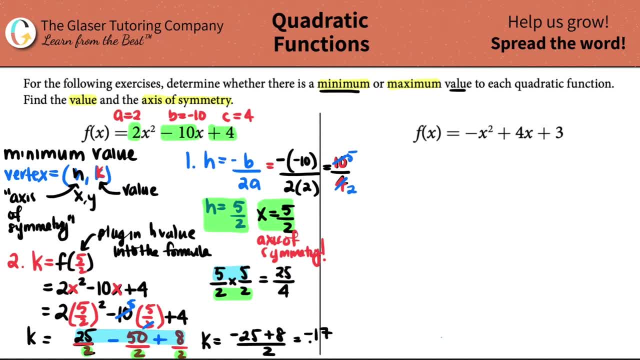 So this would be equal to negative 17 over 2.. And that is your k value, That is your minimum value. So if I just give you some context- and here is my graph again, we knew from before- the axis of symmetry was 5 over 2.. 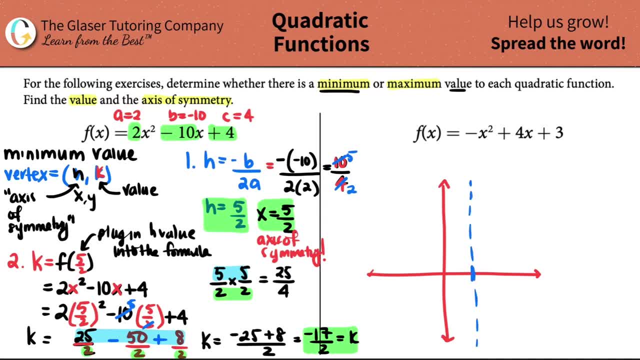 So somewhere over here, right, And my minimum value is negative: 17 over 2.. So like 16 over 2 is 8.. So like a little bit down here where the 8's are, And that's your minimum value. 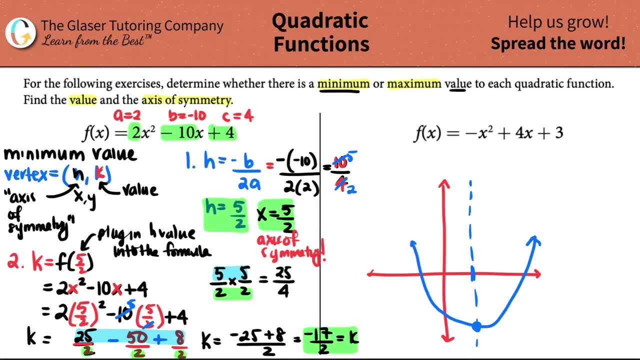 So the graph turns here right, Because this vertex would be 5 over 2 comma, negative 17 over 2.. Just to guide you, Okay, All right, So that's my graph. So that's my graph, And I'm going to give you a little context. 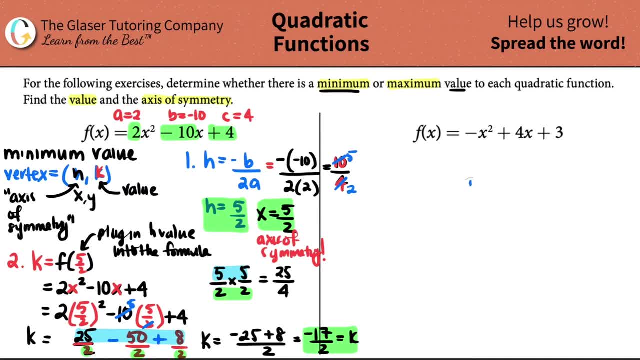 Now let's do the next one. Same idea, though, all right. So first off, let's find out if we have a min whoop. let's find out if we have a min or a max value. Remember the a value is what gives it away. 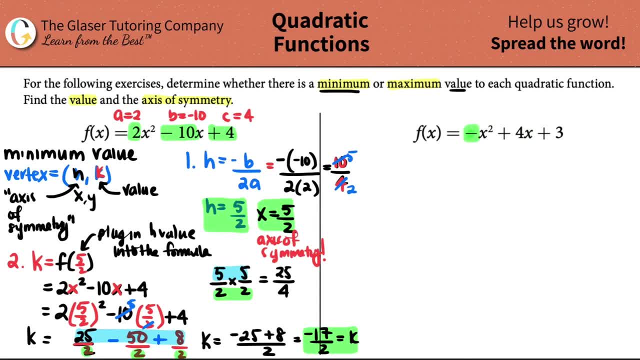 So here I just have a negative over here. right, My a value would be: what A negative 1.. If you don't have a number here, it's automatically just a 1.. So a negative 1.. And if I just go along, I have a positive 4 and I have a plus 3.. 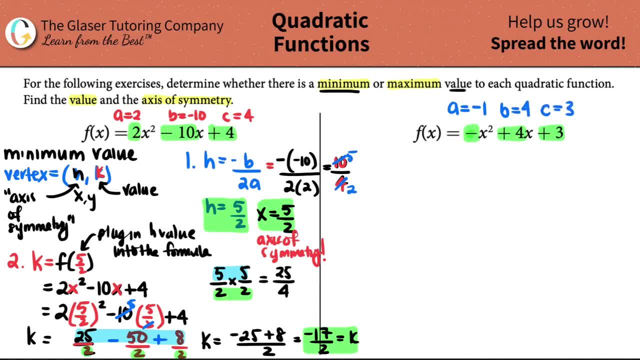 So this would be b equals 4 and c equals 3.. But I have an, a value of negative 1.. So I know that it's frowny, right? This is a frown, And frowns go with max values. 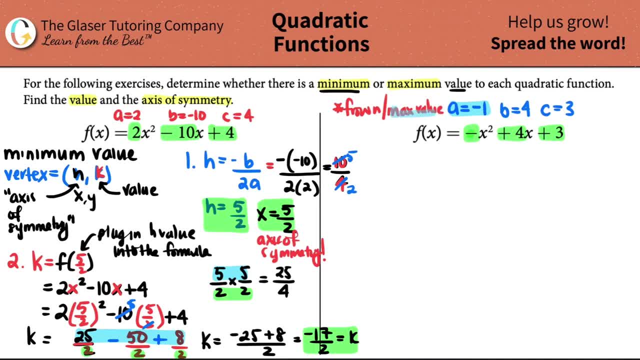 So I have a max value here, I have a maxima, or I have a maximum value. Just to give it some context. if I quickly drew this graph, I know that I have a frowny face and that vertex is the highest on the y. 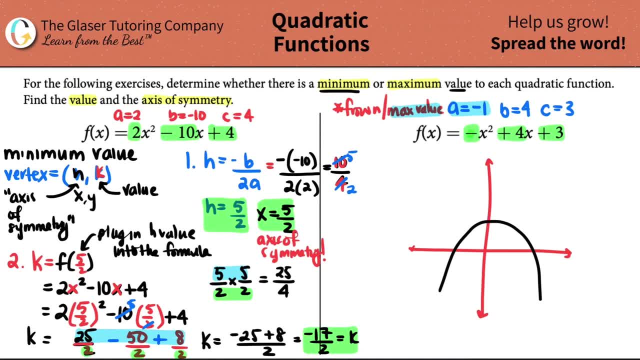 However, I don't know whether it's. you know, the intersection is here. I don't know if it's above, but I know that it has to be a frowny. If you hear the car that's blowing up, it's a BMW. 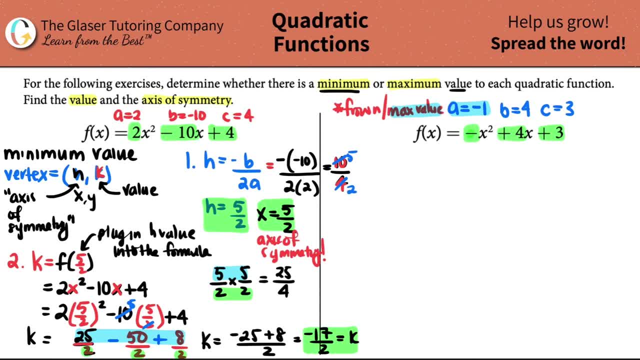 What is that called The pop, pop pops? Chances are it is a BMW. Let me know in the comments if it's a different car, but I'm pretty sure it's always a BMW. Anyway, let's keep moving. So we know that we have a frown. 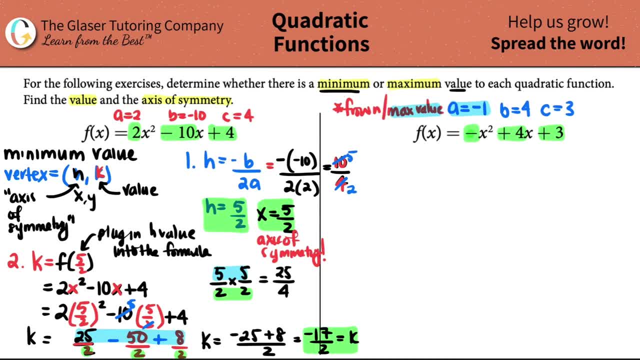 We have a max value. We need to find that number And remember it comes from the vertex. Remember the vertex is x comma y, h comma k. Axis of symmetry is the h value. The actual value is the k, But we can always find the h first. 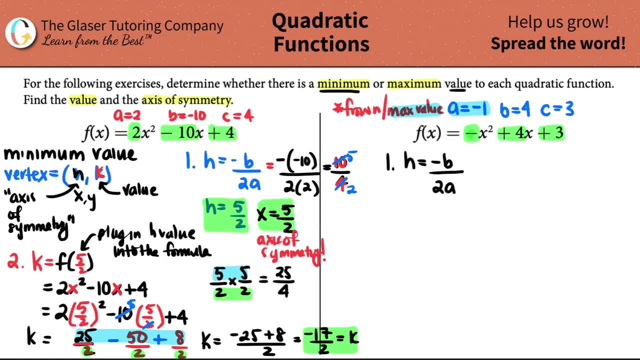 So h is always equal to negative b over 2a. We got our ab's and c's, So all we got to do is just plug it in. We have a negative 4, because that's our b value divided by 2 times a negative 1.. 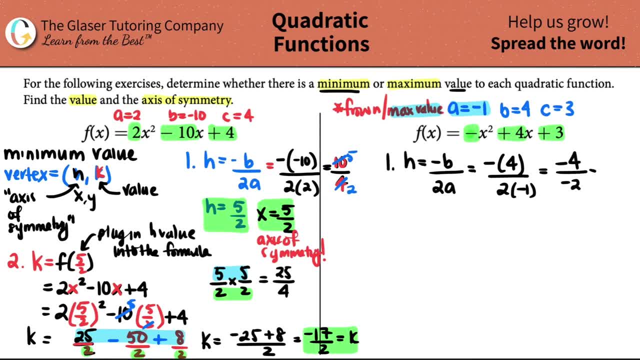 So just clean this up, I have a negative 4 divided by negative 2.. So my h value is a 2.. OK, So we answered the first piece of the puzzle. But remember, when we state that it's an axis of symmetry, I can't say h equals 2.. 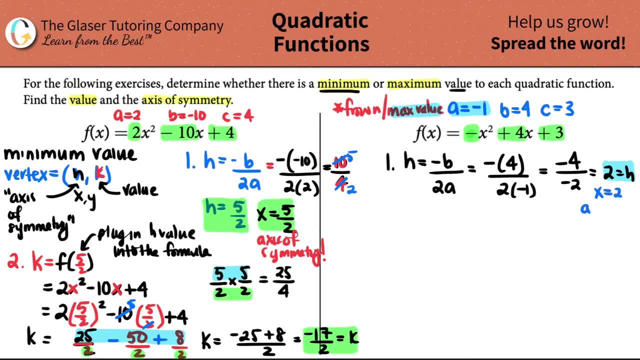 I have to say x equals 2.. That is the axis of symmetry. OK, So that's the answer to the second part. You got to find the second part, the axis of symmetry, before you get that value. So, number two: we got to find that k. 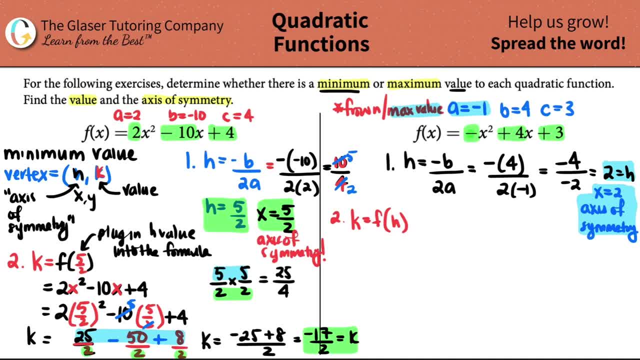 And remember k is just f of h. The h value was the 2.. So if my formula is negative- x squared plus 4x plus 3, and my h value was a 2, I'm going to plug in 2 for all of my x values. 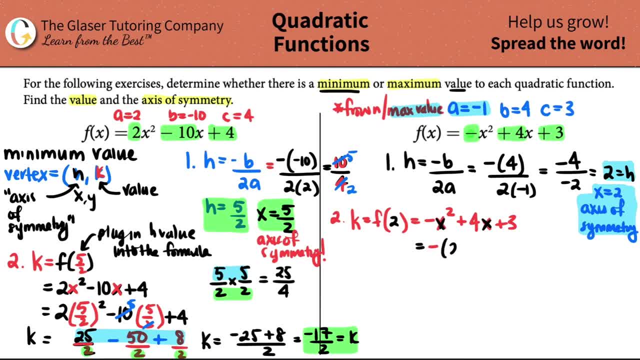 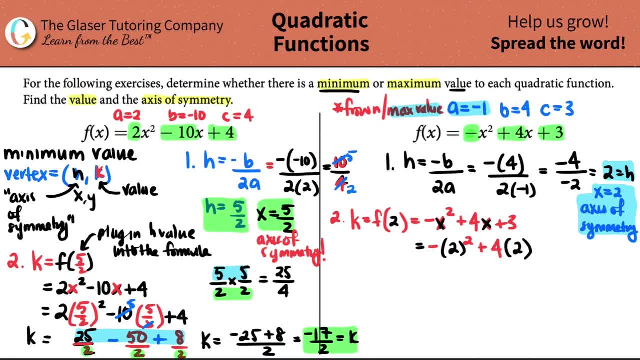 So, for example, I can get 4x2, and that's all being squared plus 4 times 2, and then plus 3.. Quickly, let's run through this math. We have: 2 times 2 is 4.. However, there's a negative out here, so it would be negative. 4 plus 4 times 2 is 8 plus. 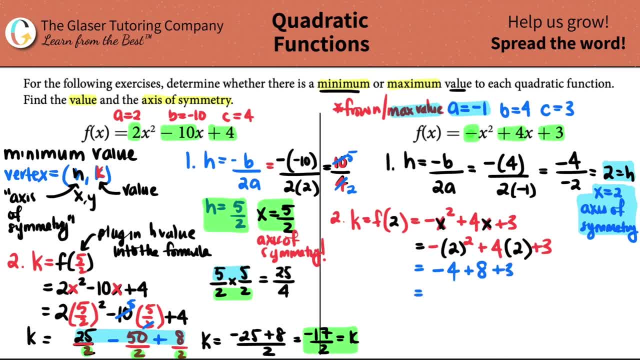 3. This is easy to simplify: right Negative: 4. four plus eight is a four plus three, which is seven, And that is my K value. And the K value is the value of the max value here, because we have a maxima or we have a maximum value. 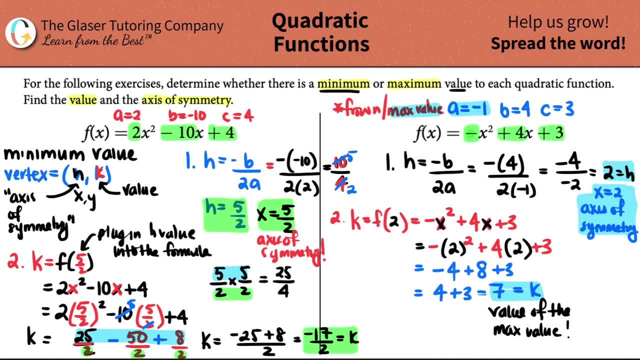 So there you go. Um guys, let me know in the comments what you thought. Give this video a thumbs up if it helped you. subscribe to the channel if you want. And yeah, I love doing these videos for you guys. I hope you guys are learning and I hope you're doing great in your 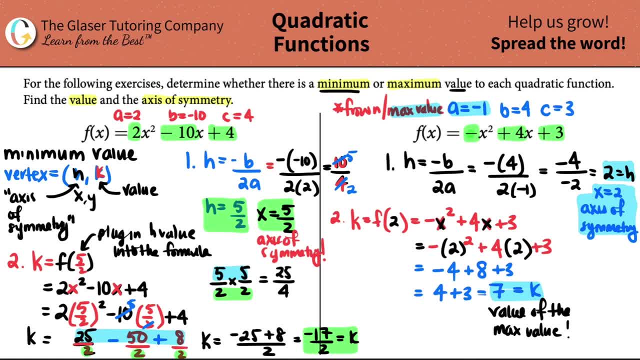 math class and all of your other classes. Um, I will see you guys all in the next video. All right, let's keep going. We love math. Well, at least I do. Yeah, that's okay. All right, I'll.